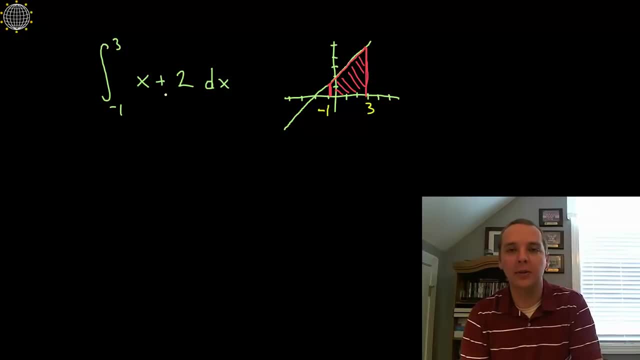 1 up to 3 right here. Now, what does this notation mean? This means the area under the curve down to the X axis or above the X axis. from my X is minus 1 to X being 3.. So we learned a great calculus way to do this in the last video called the Fundamental Theorem of Calculus. 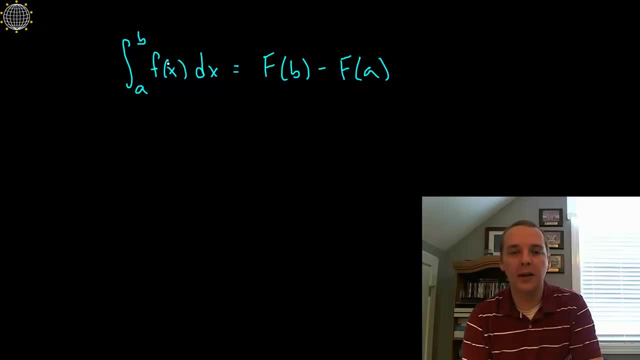 and just a quick reminder. here is what it says. in short, it says: if you want to find the area under the curve X minus 1, the area under the curve X minus 1, the area under F of X from A to B, What you have to do is find the antiderivative of little f and plug. 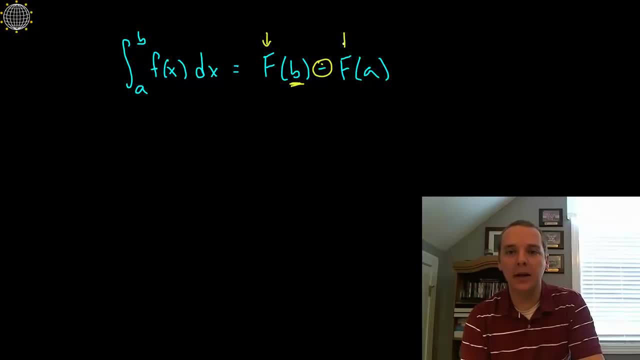 in the terminal point, minus the antiderivative of F, where you plug in the initial point and subtract those two, and then that�s the area under the curve. Okay, so let�s do that. The antiderivative of X plus 2. we can just integrate these independently, right from some. 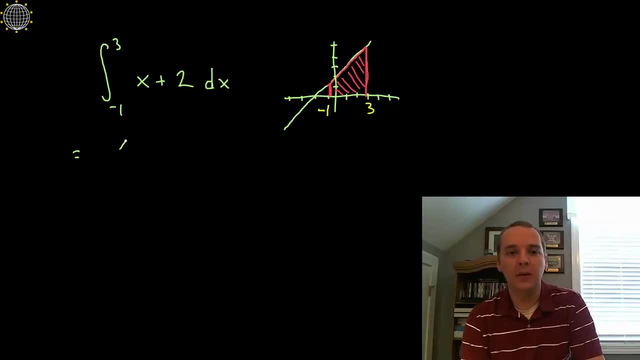 indifference rule. So the integral of X minus 1 is minus 1 and the area under the curve X minus 1 is minus 1.. The integral of X would be X squared over 2 using the power rule for integration, and the integral of 2 would be 2X for the constant rule of integration. So once you have the 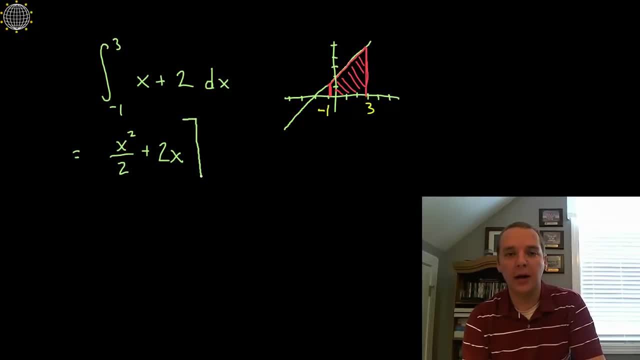 antiderivative. the common notation is: we�ll put a bracket on the right hand side with a minus 1 and a 3, and what this tells the reader is alright, in just a second, we�re going to plug in 3 and we�re going to plug in minus 1 and we�ll subtract those two. 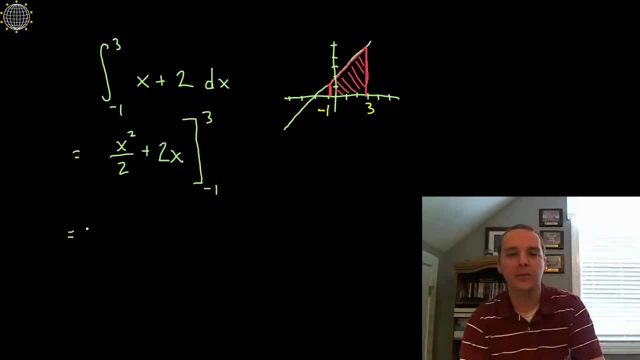 quantities. So that just keeps you from writing stuff you know all over the place. Alright, so here we go. let�s plug in 3 and then let�s plug in negative 1, and then we�ll see what two numbers we�ll get and we�ll subtract. So if you plug in a 3, let�s try to do a. 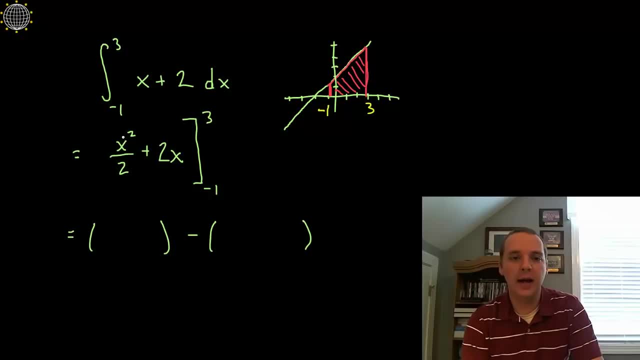 little mental math here: 3 squared is 9,, 9 over 2 would be 4.5 or 4 and a half. and then 2 times 3 is 6, so 6 and 4.5. I�ll just use decimal notations. this would be 10.5.. You. 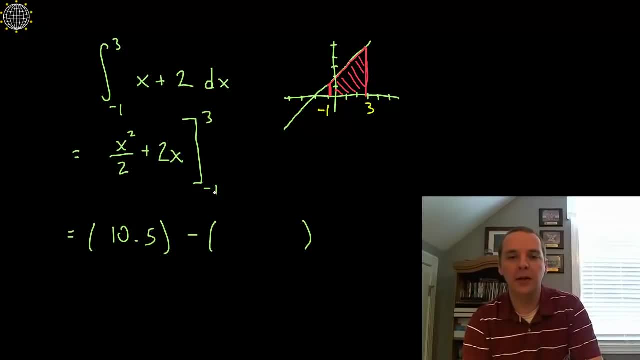 could of course write it as a fraction if you wanted to. And then if we plug in negative 1, negative 1 squared is positive. 1 divided by 2 makes a half, So we have a half minus 2, because that�s 2 times negative 1.. So a half minus 2 is negative. 3 halves negative. 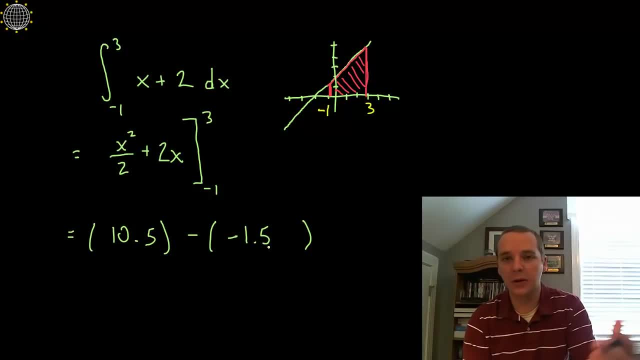 3 halves, in other words negative 1.5. if you wrote it as a decimal, but again, like you don�t have to, you could have written negative 3 halves there. Simplify this difference, and a minus and a negative will create a plus 10.5 plus 1.5 makes a total of 12. right Now? 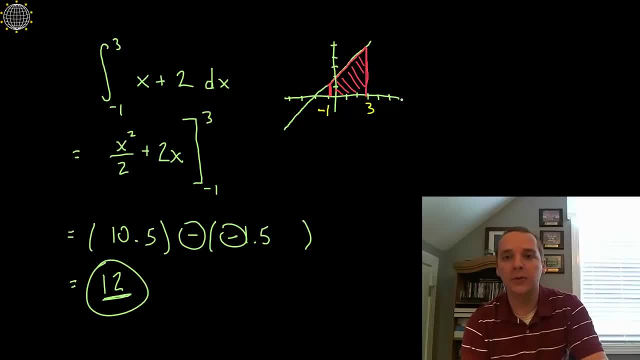 what�s 12?? Well, using the fundamental theorem of calculus, we�ve shown that the area under this curve here is a total of 12 square units of area, 12 square units of area. So if this was feet, it would be 12 square feet. if it was inches, it would be 12 square inches, etc. 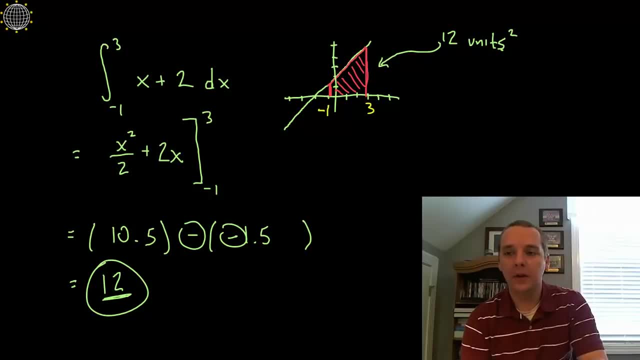 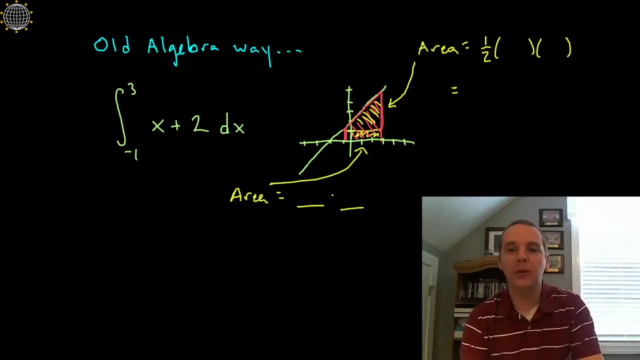 etc. But this 12 is representing area. Alright, now lets look at this the old way, just for comparison sake. Before we knew about the fundamental theorem of calculus- again, because this example is so easy- we could have done this in a round about geometrical way, just using algebra and geometry to do this. 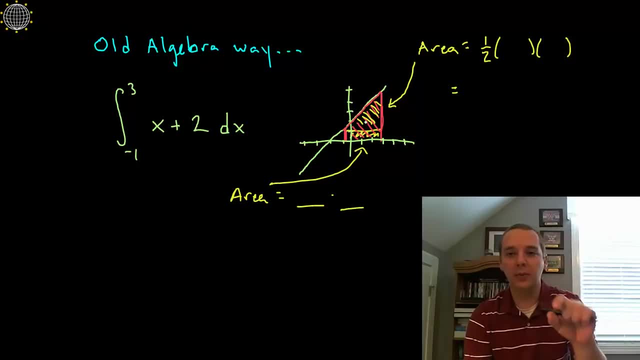 Knowing that we are looking for the area under the curve, we could have just broken this up into a rectangle and a triangle found there areas and add them together. So lets just do that real quick and just convince yourself ourselves that these numbers are going to match The area of this rectangle on the bottom. 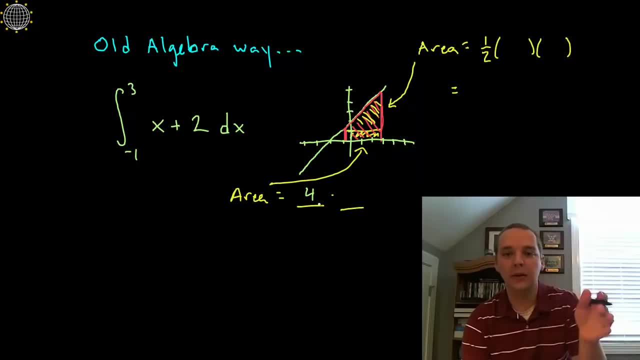 would be the width, which is four, from minus one to three, that�s the distance of four units times its height, which, if you notice this, has a height of one. and then the area of the triangle would be one half base times height. Again, the base is four and the height 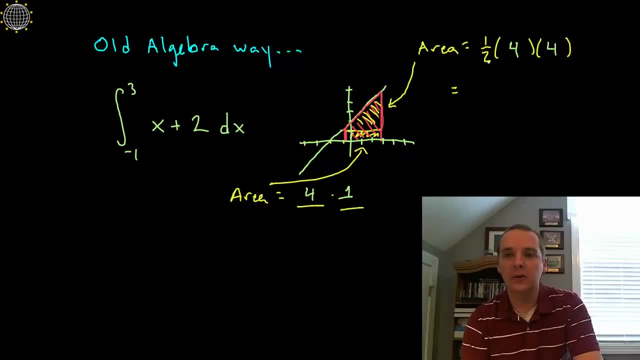 if you look at this triangle, the height is also four. So this would give you: one half times four is two, two times four makes eight and four times one is four. So if you add eight and four together, the area of the triangle and the rectangle together, we would see that 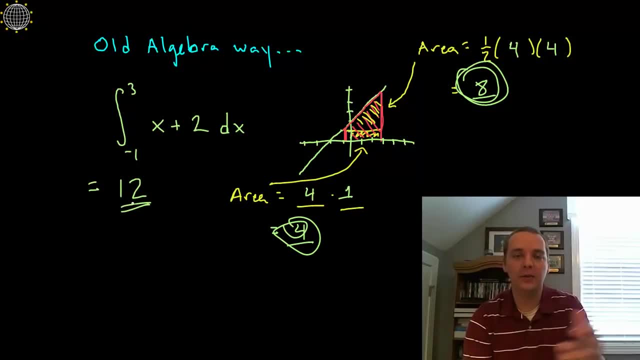 this definite integral again has an area of twelve, the same as what we got before. Now, from here on out, we�ll probably never, ever do it this way again, because this only happened. this only worked because these were nice geometrical shapes. If your function has a smooth top, 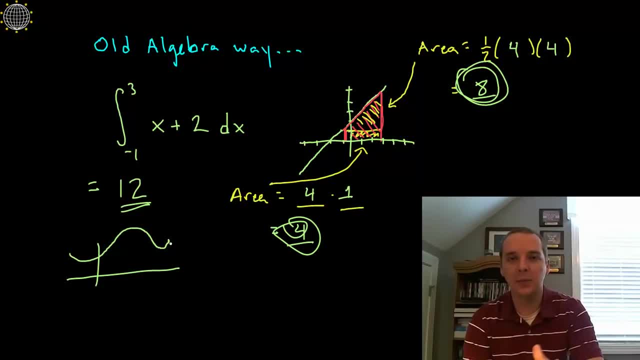 that�s curved And bending. there�s no nice geometry formulas for things that look like that, because they�re not triangles, they�re not rectangles, they�re not circles and things of that nature. So I did this just to convince you that this fundamental theorem of calculus is working. 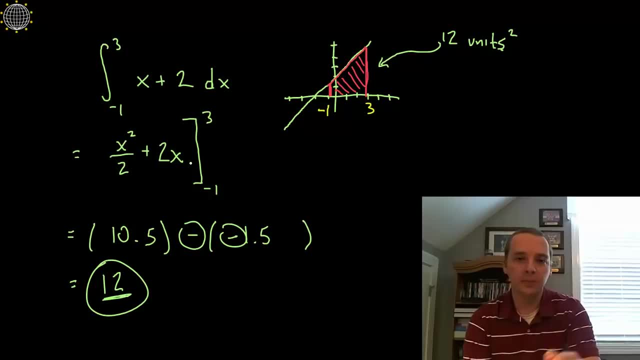 as it should, and it�s a great tool to use. So now we�ll move on and look at some more complicated examples, more on par with what you would more likely see on a homework assignment or like a test. 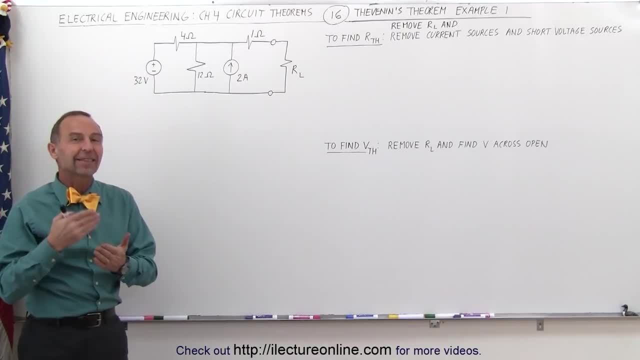 Welcome to ElectronLine. Now let's find out how to utilize that Devenin's theorem methodology to solve circuits like this. Again, they need to be linear circuits. Notice that linear circuit has a voltage source and a current source, a number of resistors, and then attached to that is the load resistor. 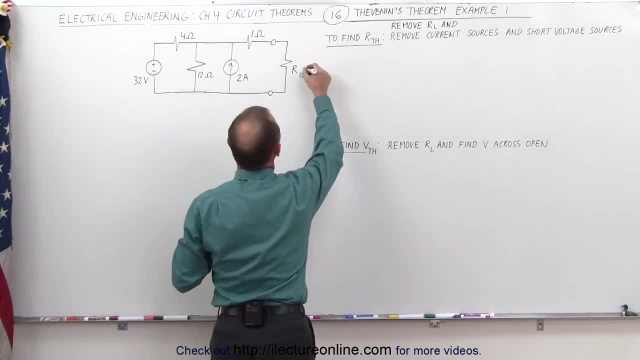 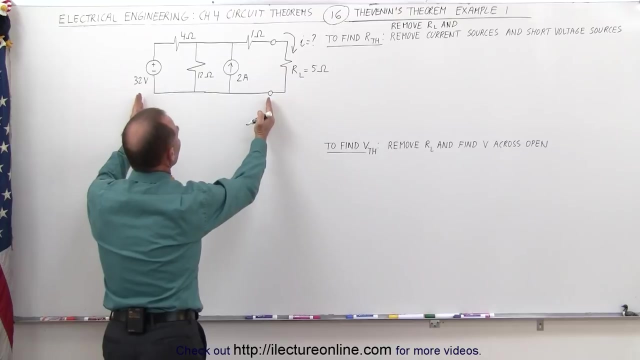 Let's say that the load resistor is equal to, let's call it, five amps, or I should say five ohms, And what we're trying to do is we're trying to find the current I through the load resistor. To do that we need to turn the circuit, the linear circuit, into a Thevenin circuit. 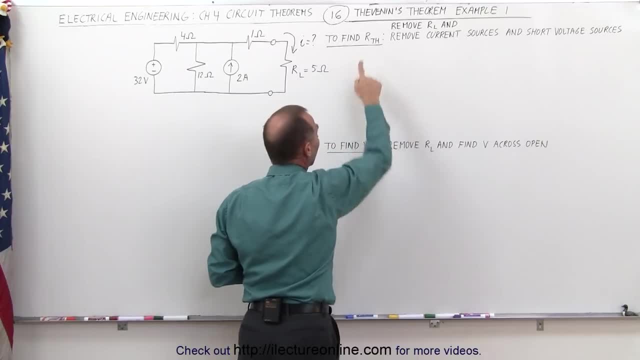 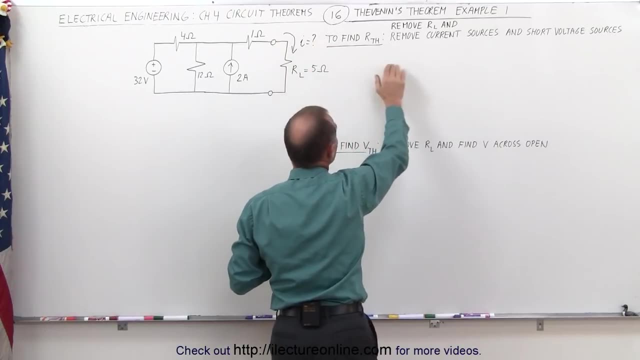 And to do that we need to find the Thevenin's resistance and the Thevenin's voltage. To find the Thevenin's resistance, we're first going to remove the load resistor and then what's remaining. we're going to remove the current source and short out the voltage source. 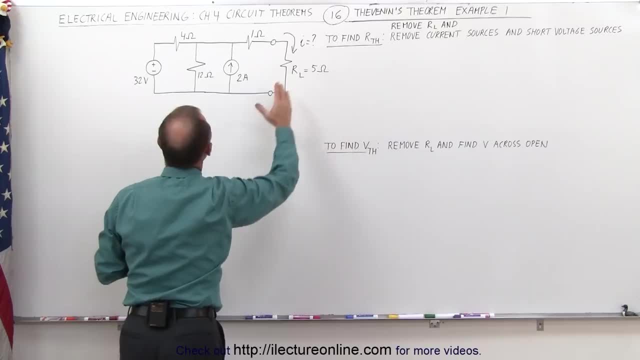 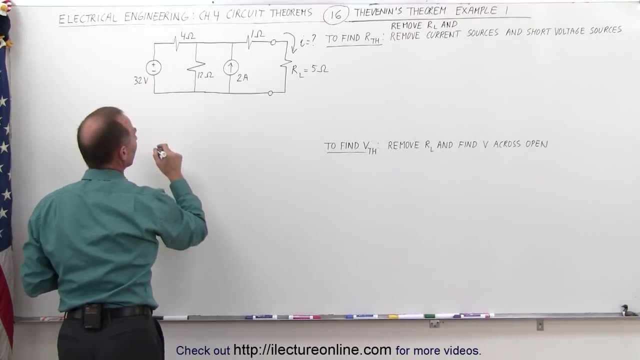 Okay, let's go ahead and do that. Remove R sub L, then we're going to take away the current source, so that will be an open, and then we'll short out the voltage source And the circuit will then look as follows: Let's put it over here. So we have a short where the voltage source was. We still have.